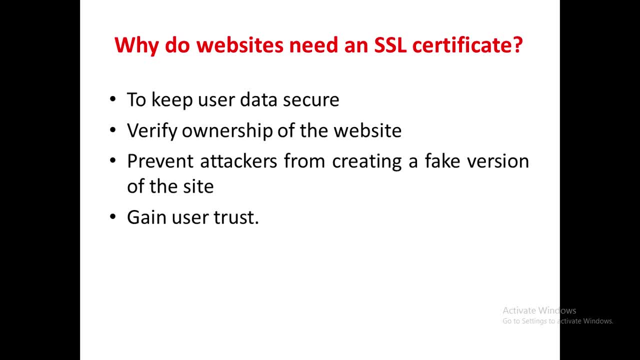 or the user will use the browser and connect to that server, so by it will give some information. is the secure information or confidential information which should not be understood by somebody, should not be received by intruder third party. but in this the hacker will create his own website of. 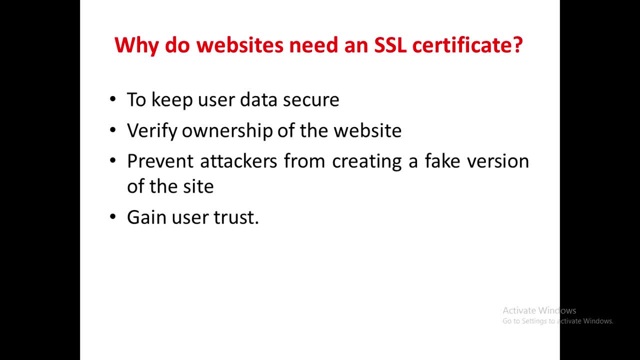 same domain name so we can't identify and we may click on it and we will submit the data. so SSL certificate will provide the solution so that what will happen if user will see that the website is secure and maybe we will see the HTTPS or the URL bar is green in color as well as it is showing some logs. so you 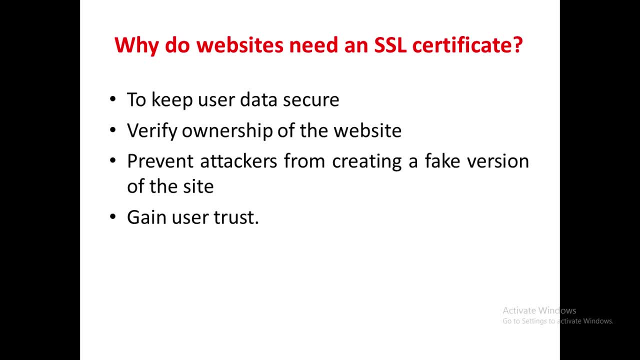 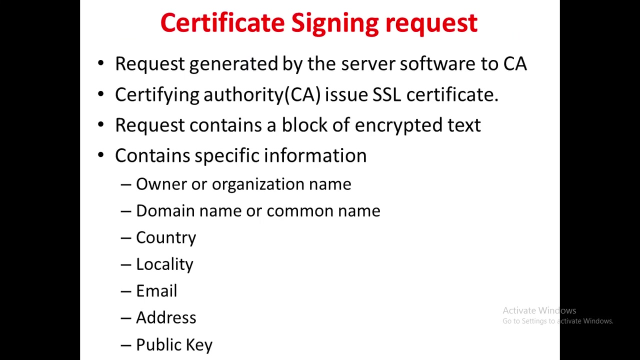 will understand that user may consider that your website is more secure. so there will be no loss of data and you can consider, as the hacking will not happen to our data, then if we want this particular certificate- because there are number of companies are there- they will provide this SSL certificate. 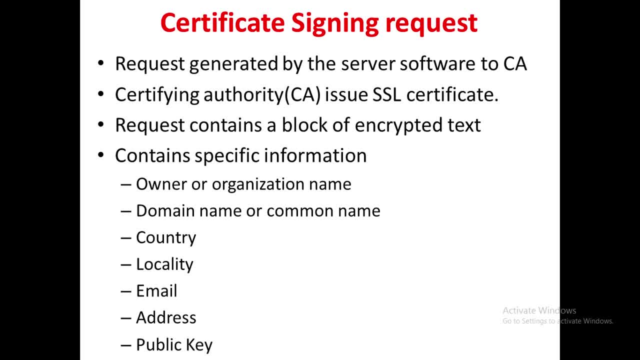 so there is some process to get the certificate from that particular authorities so we have to send the request to this particular certificate authority. that certificate authority will check our information, whatever domain name may be there, and all data. it will check and issue the SSL certificate so that, whatever we generally see what is certificate signing request, we can consider. 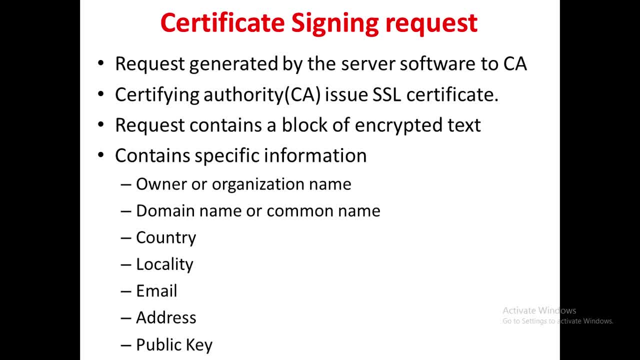 CSR by that particular client to that see, which is encrypted and which will contain the information like owner, organization. owner name is, for example, you want to make your particular website secure company's name, then what domain name you are using for that particular website that you want to secure make? 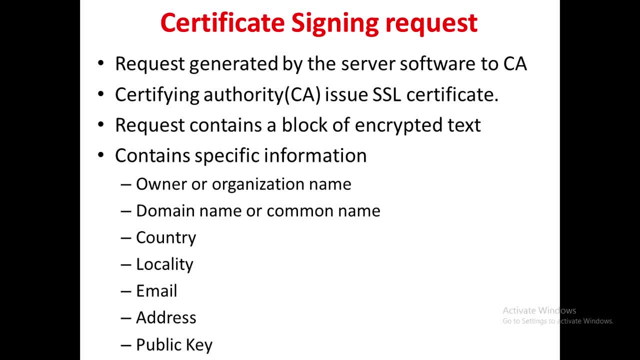 secure, then, from which country or region state you are sending this request, locality, your email, your address and you will send your public and private key will be decrypted by the particular certificate authority so that public key will be included in that certificate right. so at the time in the next, 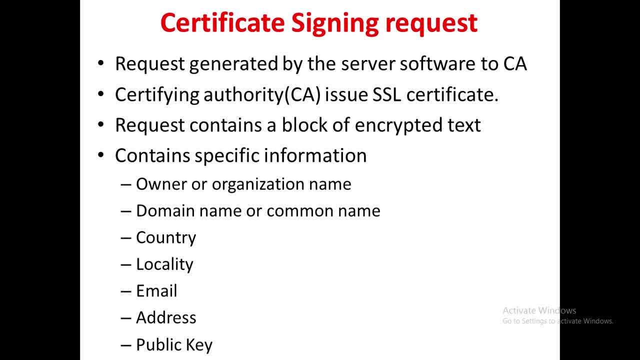 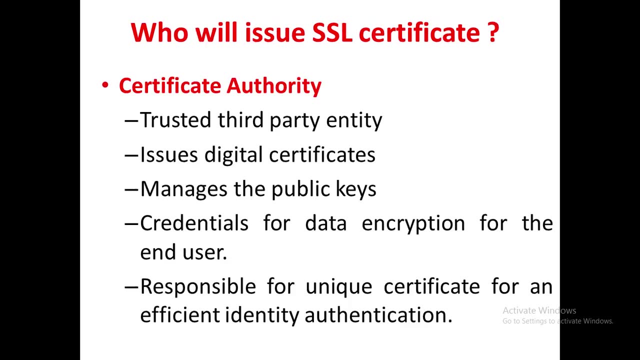 change will happen when we see the protocol. that time that particular decryption will occur by some different algorithms and we'll study. and the CSR is more important to get that particular SSL certificate from the CA. so we understood that certifying authority is what the certificate authority is used for. 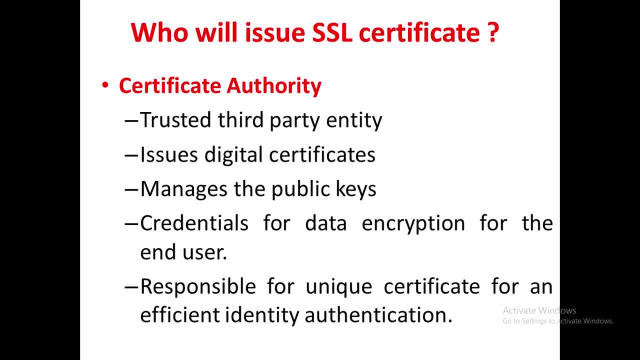 I thought it is just a third party. It is a third party. It shows the certificate, manages your public key and whatever encryptions we are using- encryptions we should use while sending and receiving the data between this browser and server- 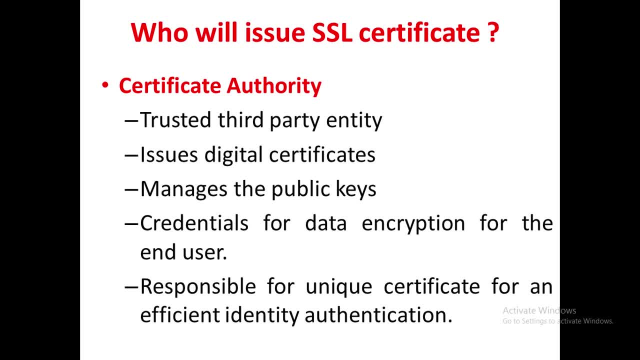 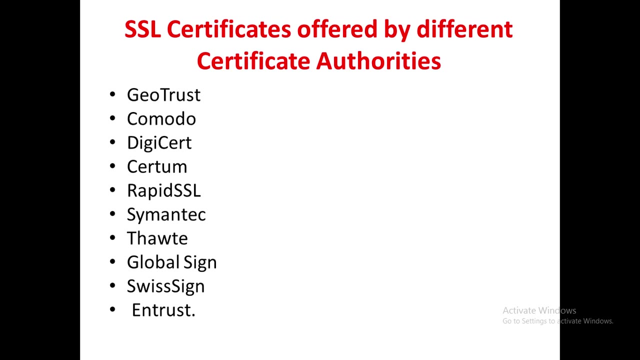 And then it will issue the unique certificate, which should not be again. you can consider the domain name. whatever we assign, that domain name should not be again replicated or it should not be again given the same domain name to the other person. So that is also important. So the certificate is very important. in the SSL certificate issue. There are a number of authorities are there who will issue this by taking some data. 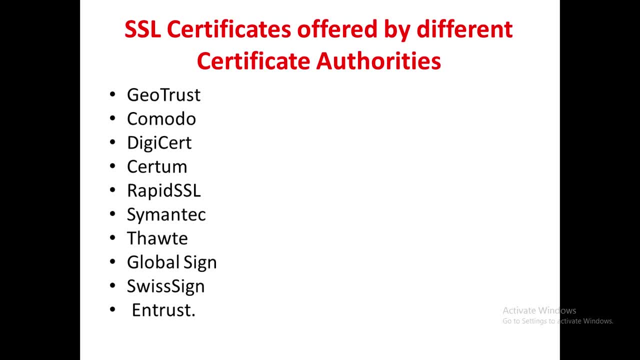 Some charges yearly, one year, two year, three year. So according to that, they will charge you and they will provide that for the SSL certificate. So there are a number of authorities like GeoTrust, Komodo, DGT certificates, Certum, RapidSSL, Semantic, GlobalSign, Sign and Trust. 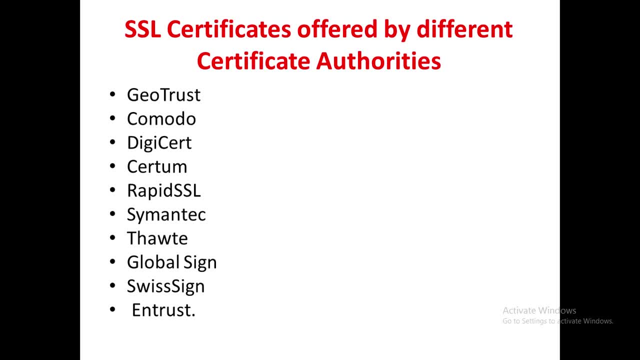 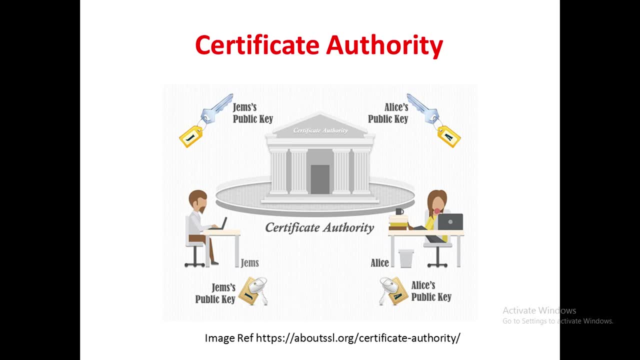 Like this number of authorities are there, they will issue this particular certificate. So this is what we can consider as the certifying authority where these two public keys which are generated and which are then considered as they are inserted into our certificate by that particular certifying authority. 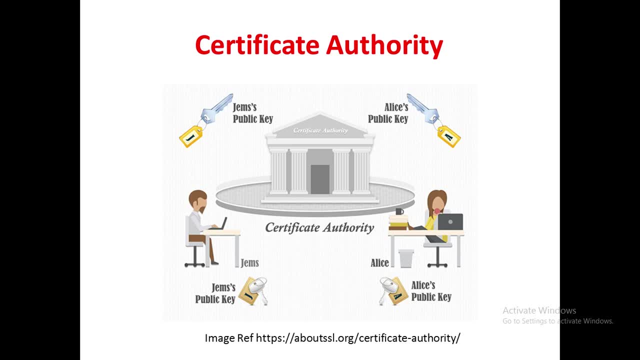 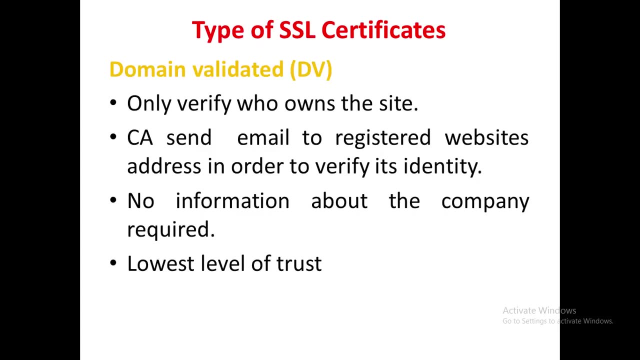 So at the time of communication between the AND user and your server, so this decryption will occur. Then, when we go into the detail that different types of SSL certificates are issued by these authorities, it is not like that once what type of level of security you want from this SSL certificate. 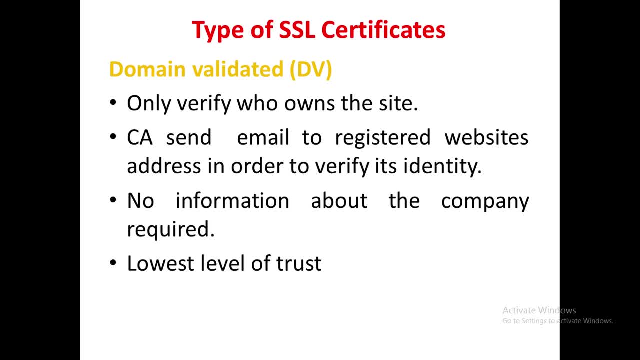 So according to that, the certificates are issued. If you see that the first one is a domain validated, It is again the lowest level of trust where it will see that the domain name should be unique and it will see that you can verify the owner's site and issue that particular SSL certificate to that particular company related to that, only for domain. 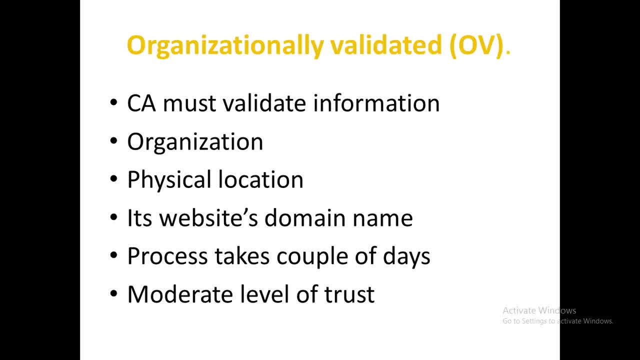 We can consider that Then. second one is organizationally. It is the second again. second level of certificate is issued to the company that here some more information is validated like certify authority. it will check your information Like organization, your location of company, then your domain name. 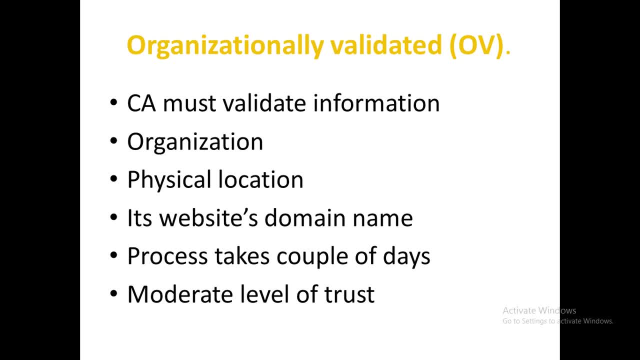 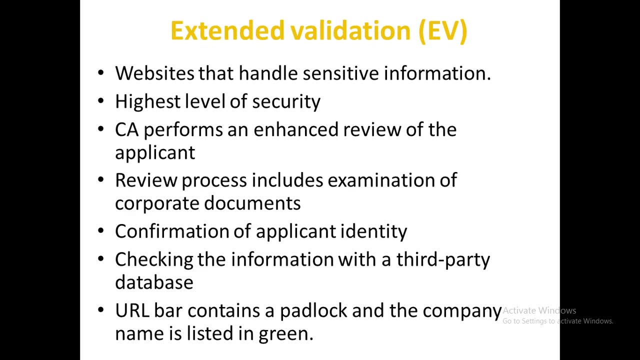 So it is somewhat again, take a time, because at this level they will check at some more deeper level to give you that particular organization validated certificate. So this is the second level of certificate And this is the third level of certificate where extended validation. 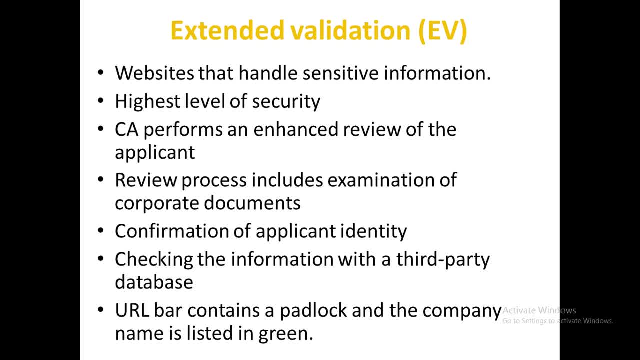 Extended validation is the most you can consider the highest level of certification. Extended validation is the most you can consider the highest level of certification. Etc: Extended validation is the most you can consider the highest level of certification. Extended validation is the most you can consider the highest level of certification. 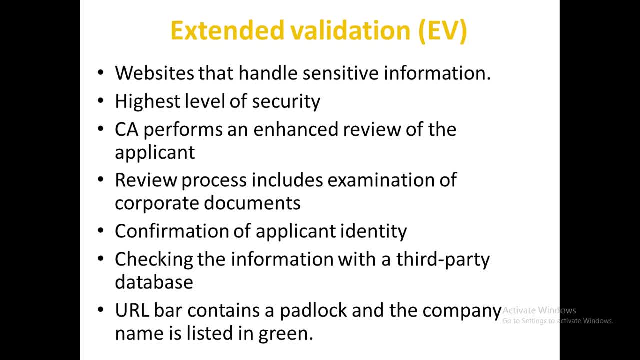 delighted. Then this third is the second low level of certification. Ordered hardships, Res, sunshine to schedule period, Sorting by看一下 activity sequence or defining series. This finish, provide the ideal level of your certificate, is a crucial requirement for your project capitalization. 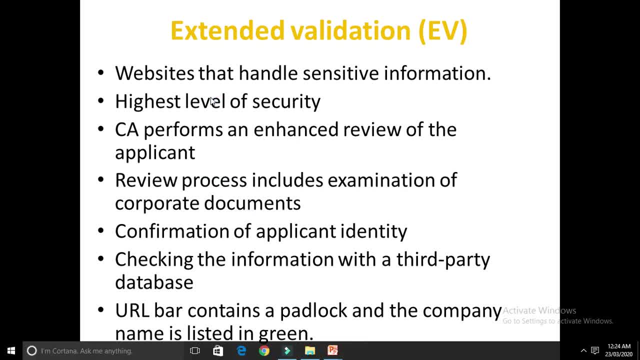 These qualities of the landing page That will be your personal key that the blogger can access and it will also give their千 and squaring funding. All reach their goals, and goals done at low zeal for ИП, where you can get your certificate in a BRUH doubts authority for success. 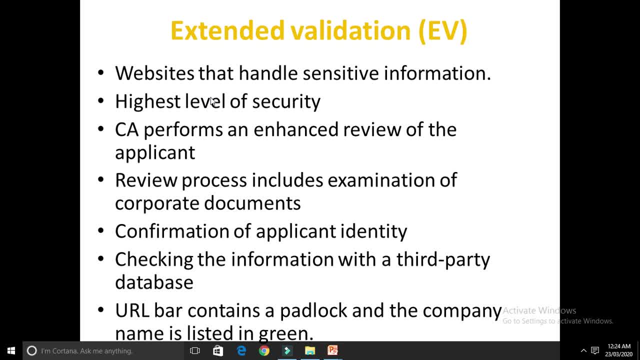 There are many license to avoid other terms of � Join the community besides register at the bottom of it is a system within the login circuit. so they will check in their database also related to your company as well as related to your domain name every information so you can see that the URL 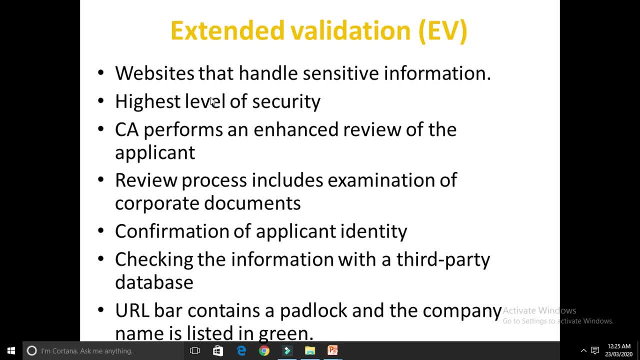 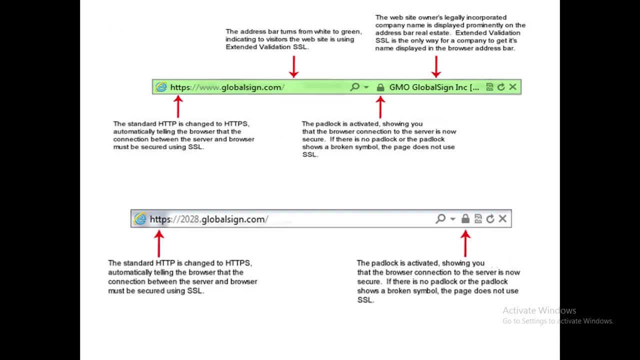 bar will contain the lock and company's name is listed in a green color. so this is also one extended validation. you can see that in our SSL set word issue. so if you look at this images, you can find where, instead of HTTP to HTTPS, yes will specify that it has to the certificate related to this domain name. so it is a. 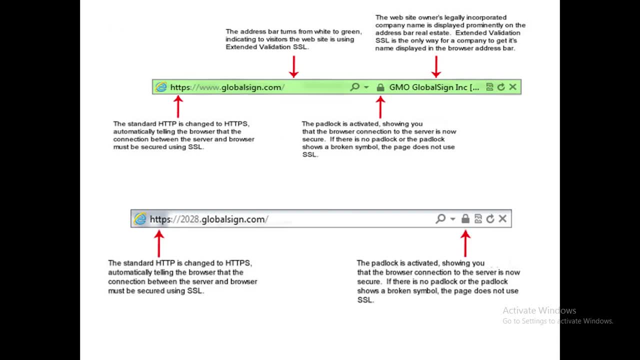 secure compared to HTTP. then another: you can find this particular lock we can find here. this lock will also show that your, whatever getting that, a checking the getting that information from that website, that website is not fake, it is secure, and then you can see that a green light. we. 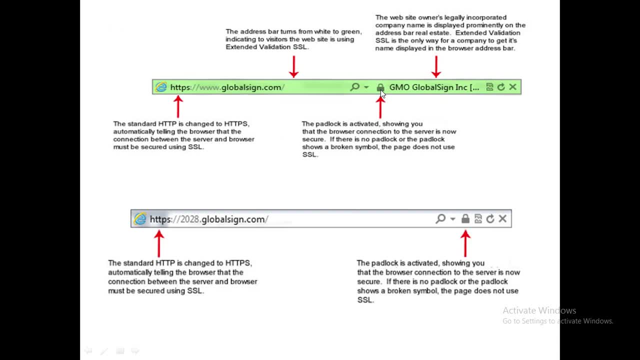 can find. this is also one way to show that it is a secure and sometimes in extended validation you can see that sometimes in extended validation it will give the company name also on that particular URL. so like this, some more security is we. we can see whenever we open in the browser. so if we have this HTTPS or lock, 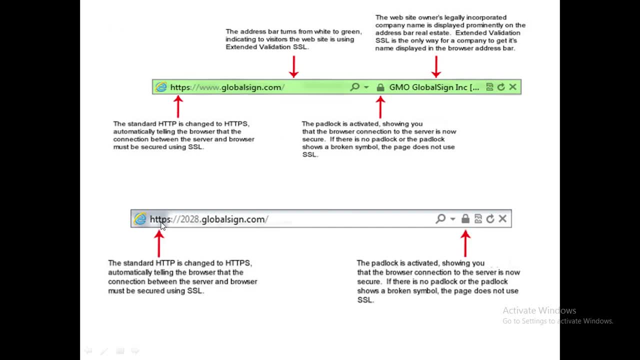 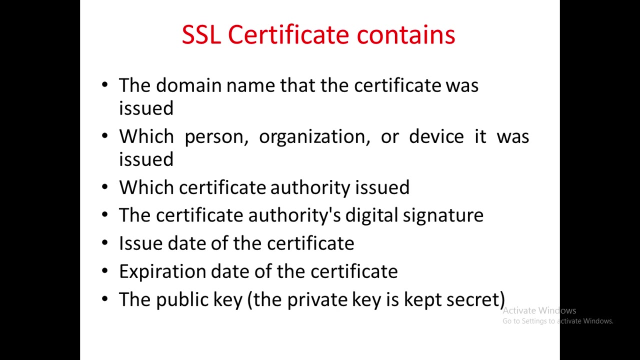 or this particular company name with green color by URL bar. so we should consider that the website is more secure as well as authenticated website so we can find. so once the SSL certificate is issued to that particular client, so he will install that particular in his iander search traffic for the next. 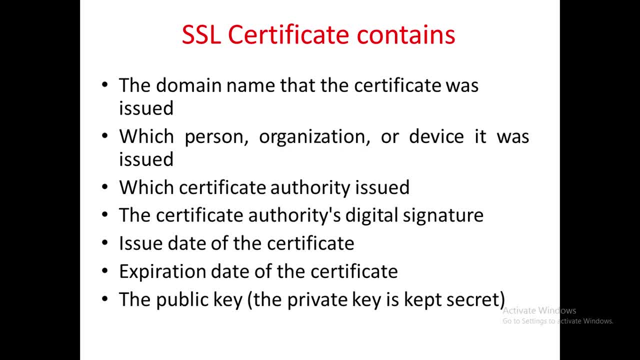 startup server that particular certificate child server into the web server and when we will obtain now that particular certificate, he to give some files and then will run that files, download that file on his web server and the people in that particular one is certified, so that this is a template that contains a person or an organization to which e issued to divide and it's who can be.